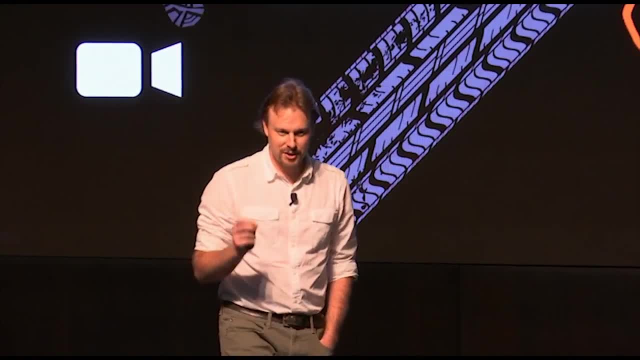 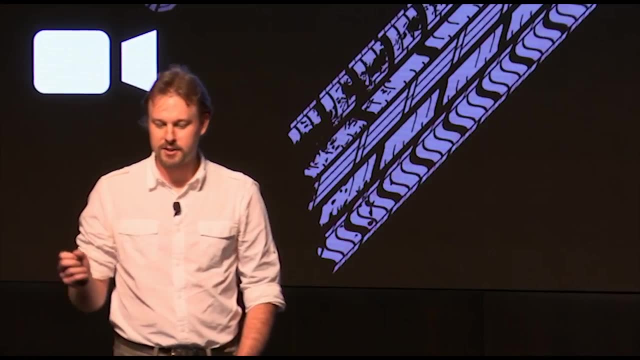 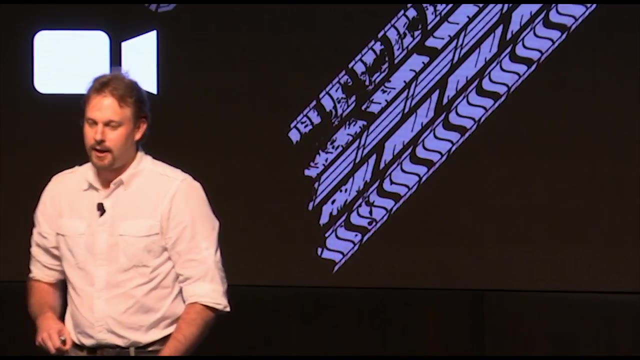 is called proxies. Proxies are really important, and so we use them in a lot of different ways, and you can see it based on the slides. We use things like DNA evidence, fingerprints, sometimes video recordings, tire tracks, sometimes geochemical evidence, And so we use these. 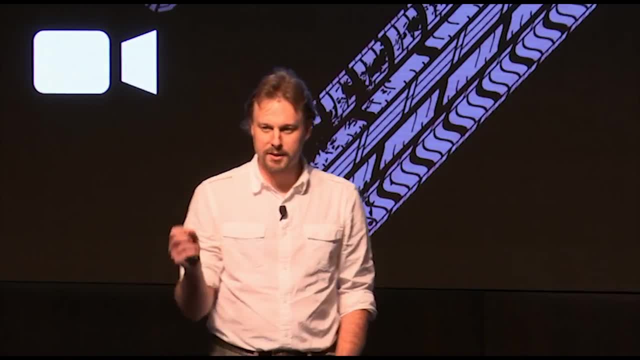 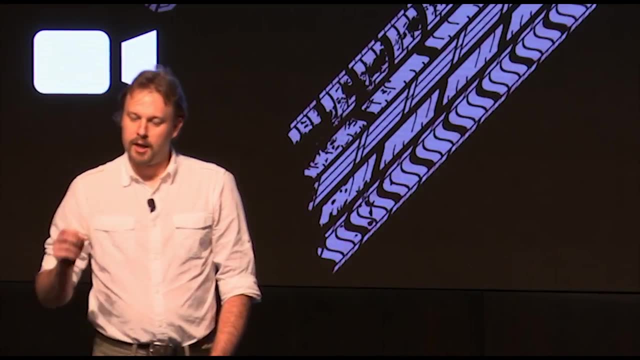 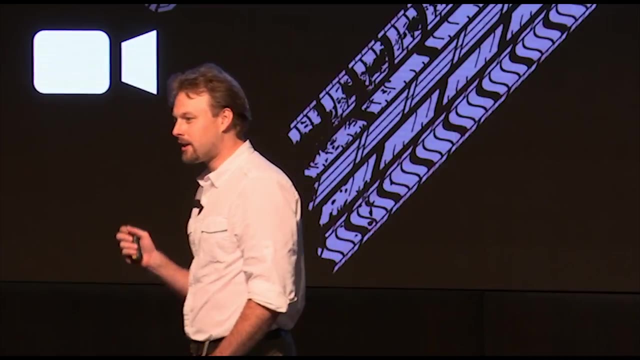 proxies to understand who might have been there and what they might have done and sort of recreate a line of thinking of what might have happened. right, And this is exactly the same thing we do when we try to reconstruct climate. And so proxies are exactly what we use. Some of them are very similar. proxies use similar machines. 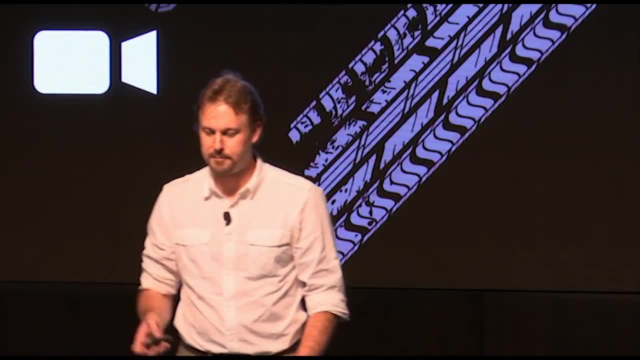 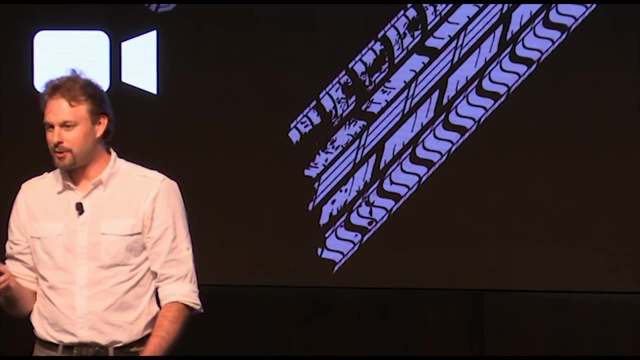 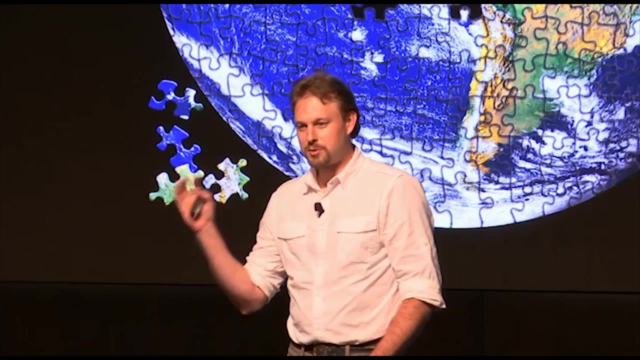 even, but we reconstruct climate using these proxies and proxy data. So I want to show you guys today how we some of the aspects of how we do this and the puzzle that we're trying to recreate or reconstruct in our record And so you can think of the earth as one big 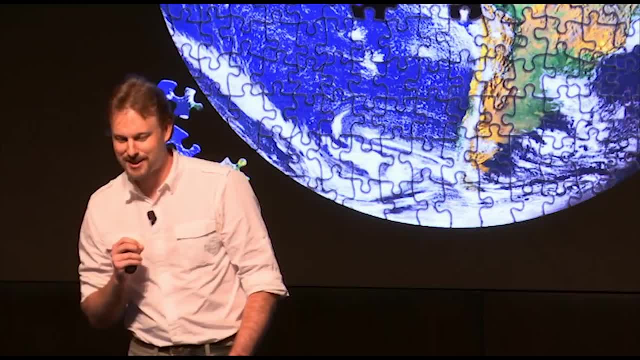 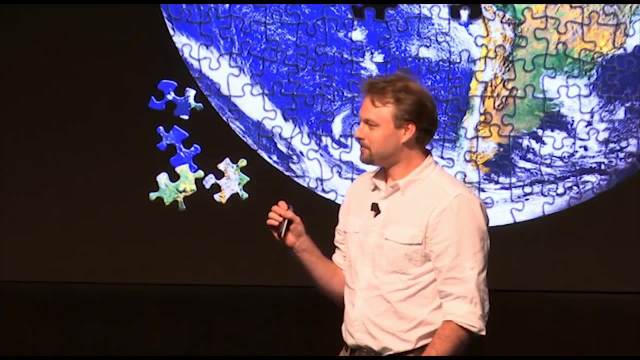 puzzle and many puzzle pieces- right, There's far too many pieces here to count- and we're trying to recreate what that climate might have looked like In the modern record. that is relatively easy. I say relatively because it's easier than time periods of the ancient. 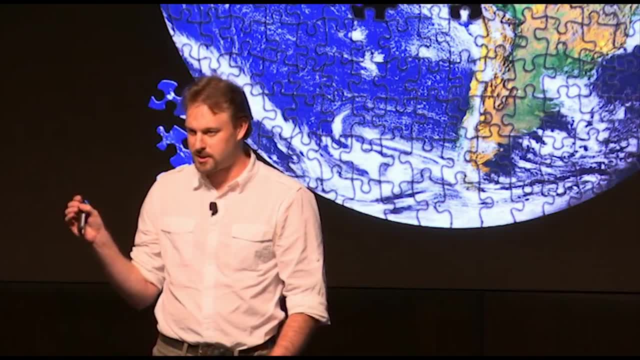 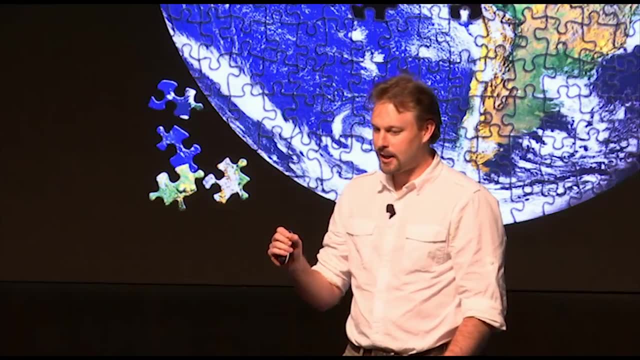 record, And so there might be either fewer pieces or less pieces missing, but we can put together and piece together the climate record, And so what we're trying to do is use these different lines of evidence and proxies to reconstruct that climate. Some pieces are more important. 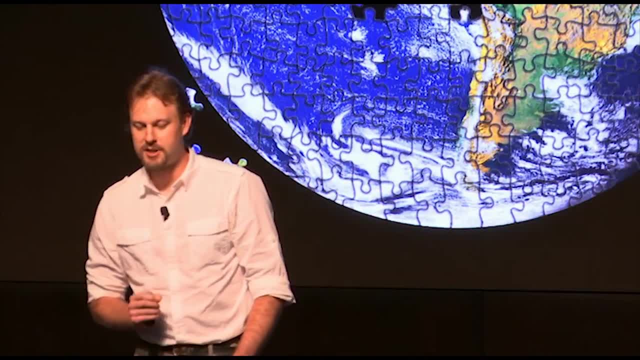 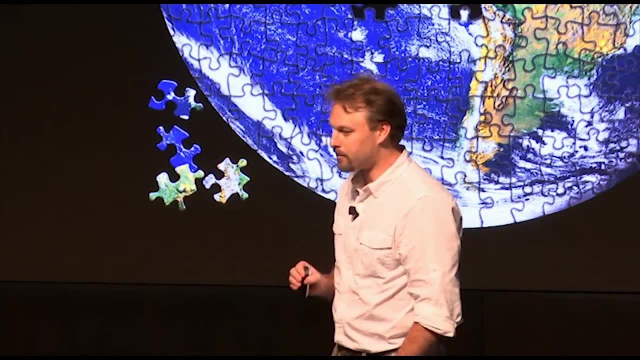 Some pieces, like off the east coast of Brazil. here you can see that you don't know if that might be an ocean that fills in and so you have an island next to it, or if it's, the entire continent is filled in, And so some pieces of the puzzle are more important than others. 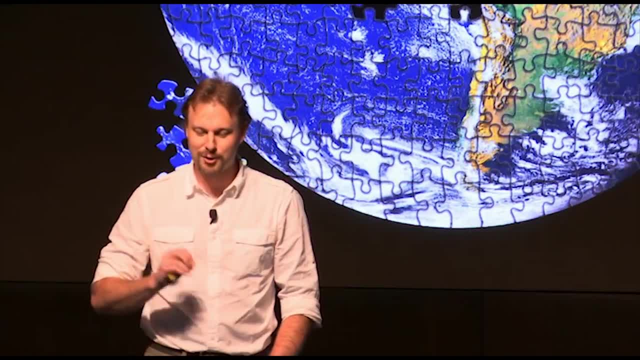 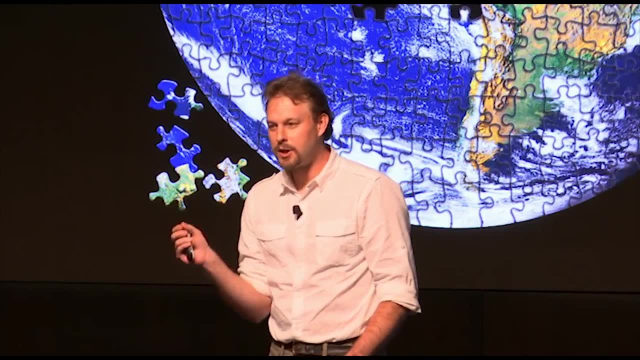 Sometimes we fill in the puzzle incorrectly, like if you were doing any large puzzle and they have the same colors, like blue ocean, throughout. you'll probably put them in the wrong places And we do that in science. but we go back and recreate that and reconstruct. 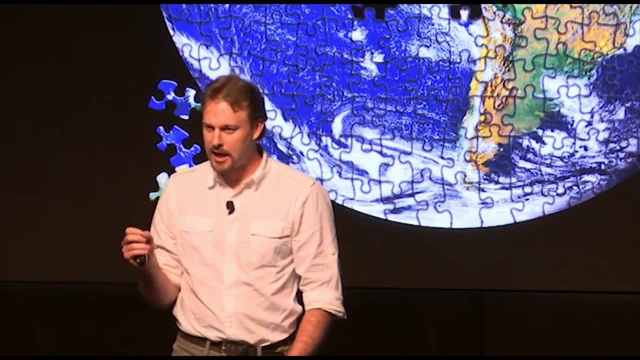 it and fix some of those things, And we're putting those pieces together And so we're trying to recreate that and reconstruct it and fix some of those things, and we're putting those pieces together And so over time we're getting a much better and clearer vision of what the climate has. 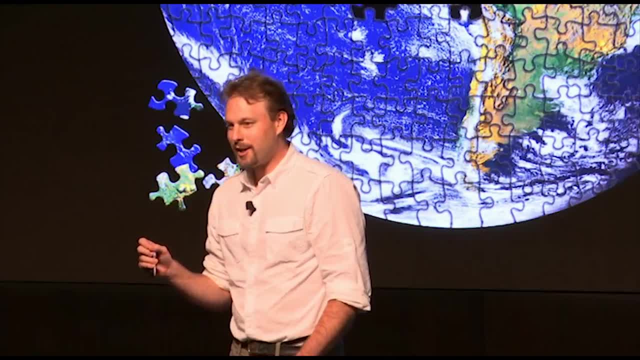 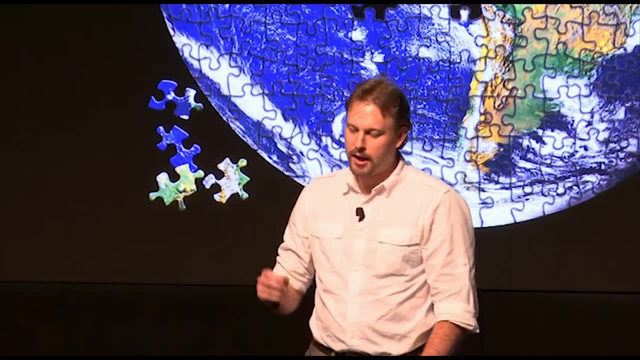 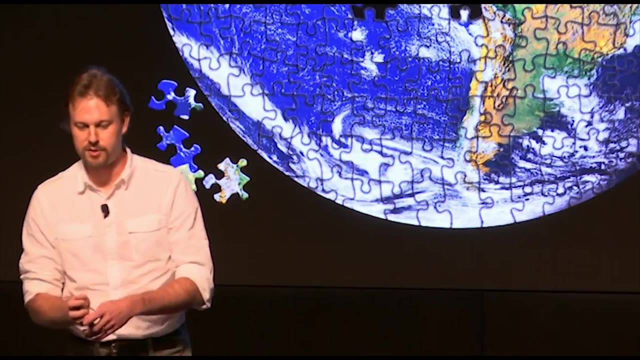 looked like. So in the modern record we can use things like instrumental records right, We can measure the CO2 in our atmosphere and we've been doing this for about 60 years, And we know that CO2 in the atmosphere is increasing dramatically. It's increasing by about 100 ppm over 60 years. 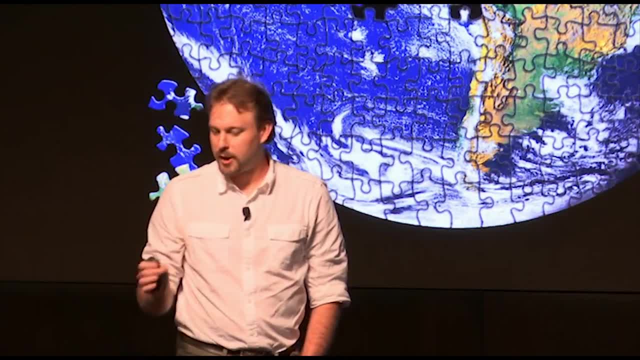 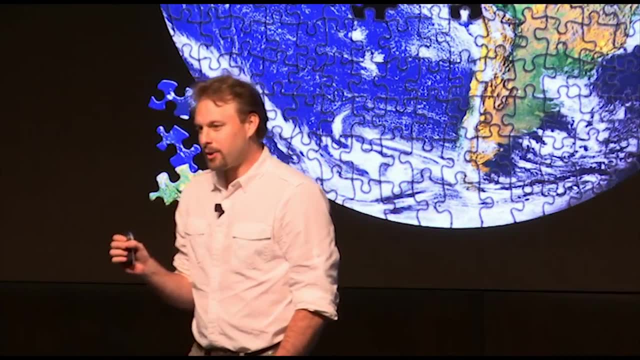 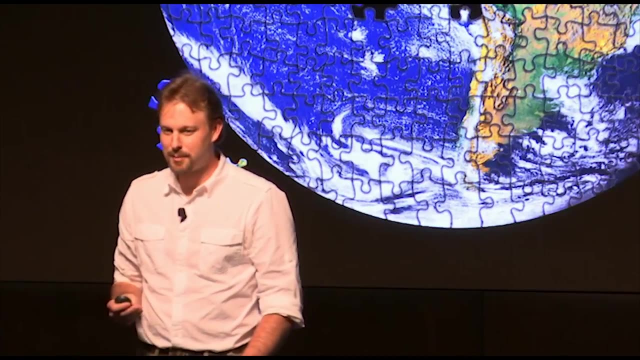 which is very, very significant, And so this is one way to do it, and we have instrumental records that go back about 150 years. We also have anecdotal evidence from people's diaries and things that can go back a little farther than that human history. But after that, what do we use to be able to reconstruct? 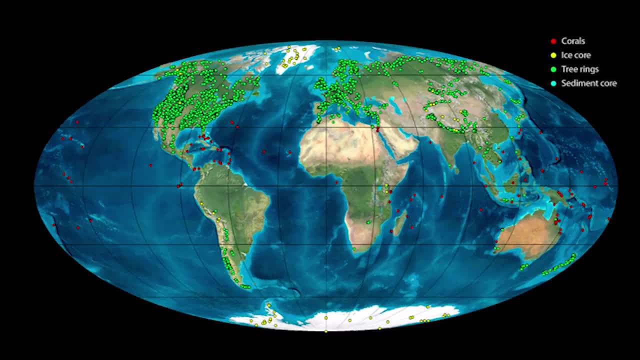 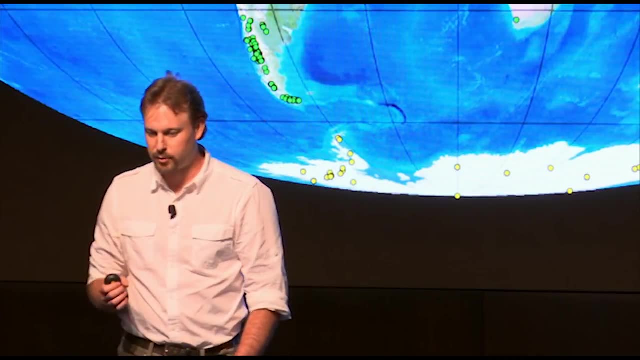 climate, And that's a really big, important factor. And so, to do that, what we actually use here is various different proxies to fill in those pieces of the puzzle, And so one piece of the puzzle would be something like the tree rings, which is, the green dots in. 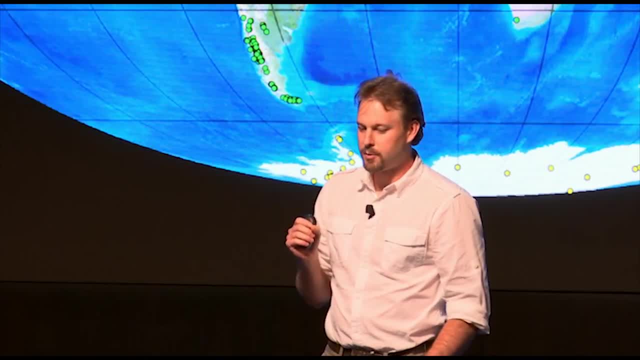 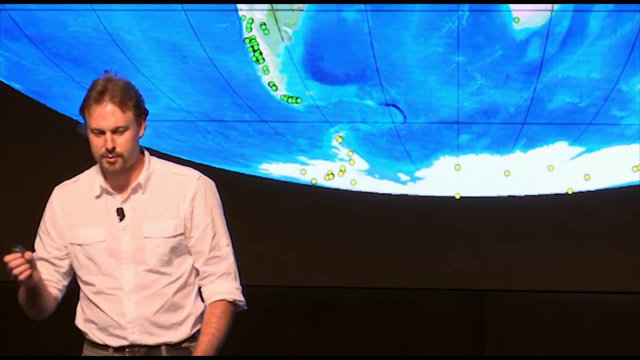 this And you can see quite a lot of green dots. These green dots are representing the tree, representing where we have tree records from, And you can probably have made out at this point that these are in our temperate regions, right? These are places in those. 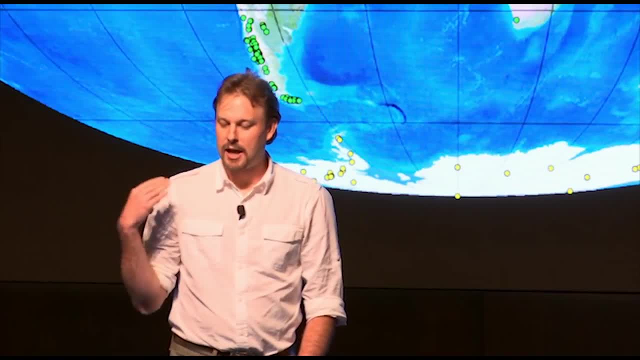 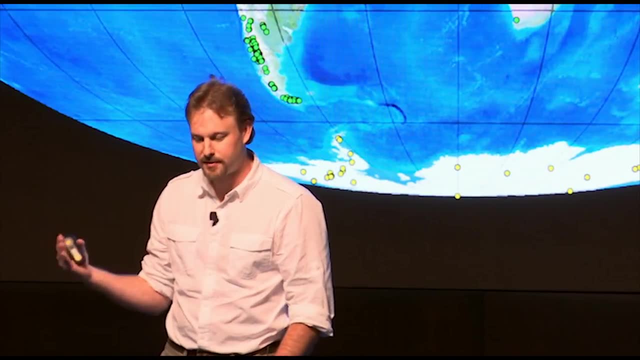 sort of mid-latitudes, And these have records that have seasonality and that's why they only exist in that area. They're very good records, but they only go back until the last living tree, which is a few tens of thousands of years. 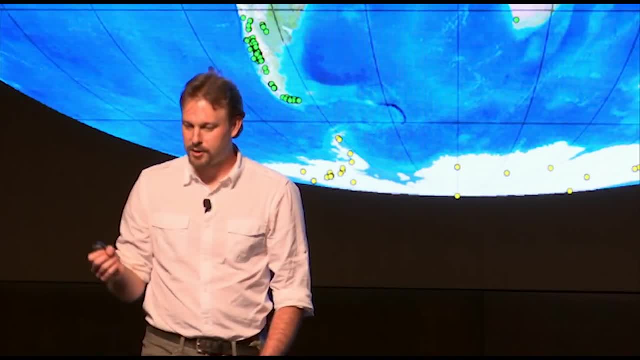 Other records might be ice core records, which many of us have heard about, And those are the yellow dots here, and those are in our polar regions And so they give you a piece of the puzzle in that polar region And those go back about a million years. 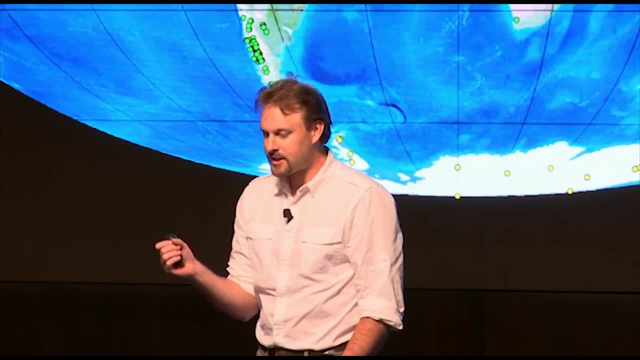 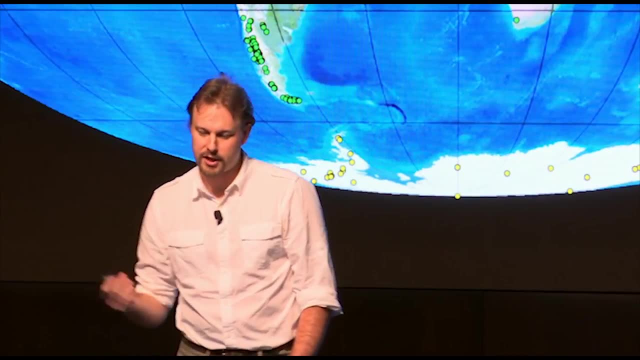 Other lines of evidence might be corals, And so corals in these red dots where you can see that they're in the equatorial regions give us very good records of the equator, And they'll go back a little bit farther, maybe two or three million years at times. 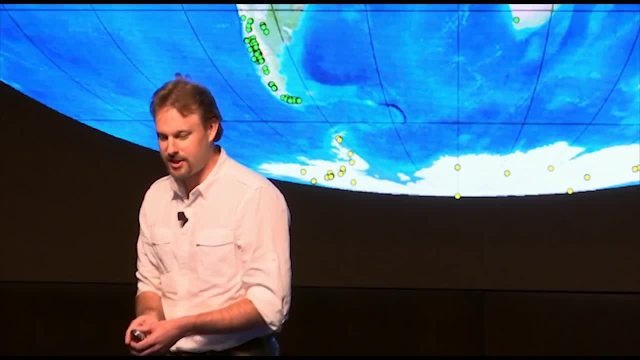 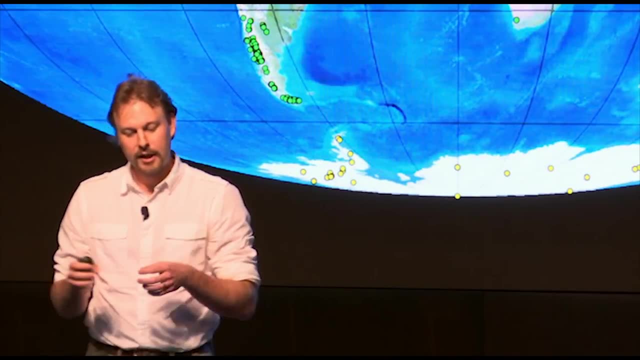 And so it doesn't go back all of Earth's history. So to reconstruct the entire Earth's history we have to use other lines of evidence, And these all have strengths and weaknesses. They all fit pieces of the puzzle and they're different. And so when we look at sediments, 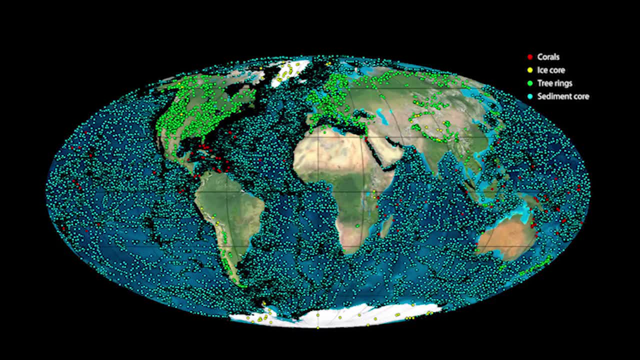 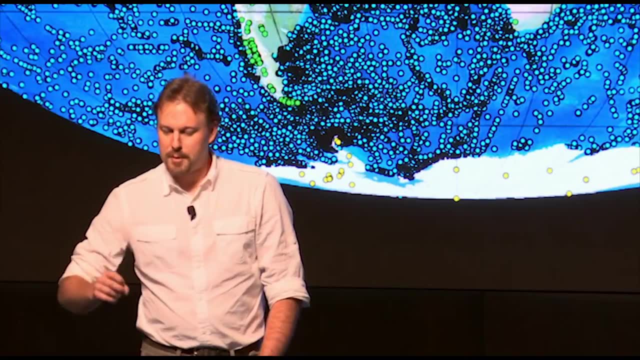 you can see that we have lots of sediments all over the ocean And it makes up a lot. Like I said, they're all pieces of the puzzle And so there's strengths and weaknesses with them, And so when we look at these sediments, these sediments are something that we're trying. 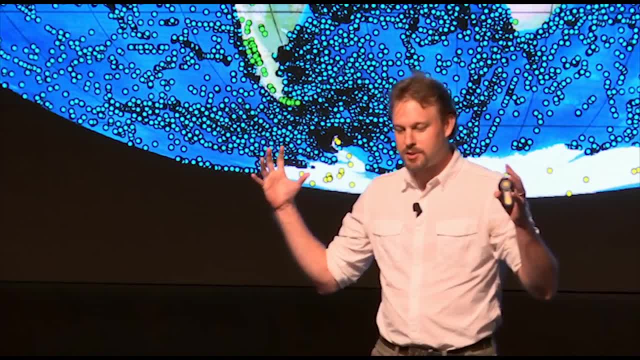 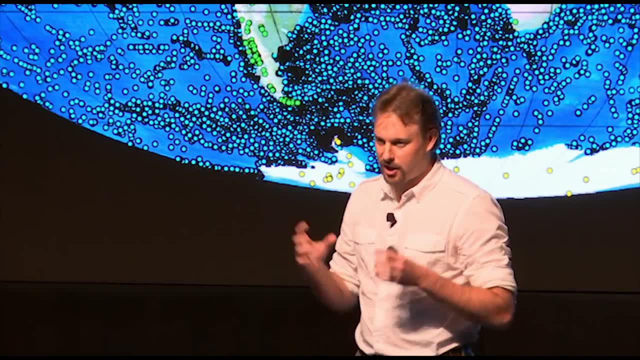 to relate when we're talking about climate is we have to unify different parts of science, which equals taking and integrating physics and chemistry and biology all in one to better understand the system, And so it really takes a large team and a large amount of people. 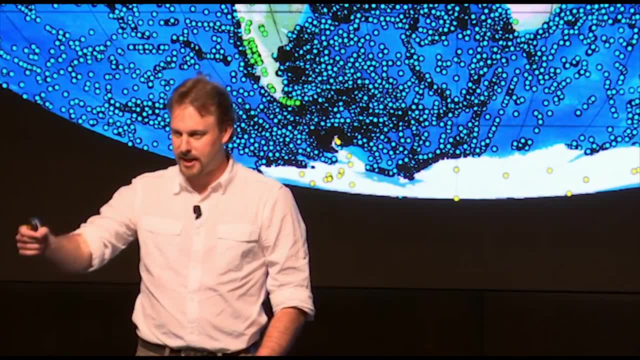 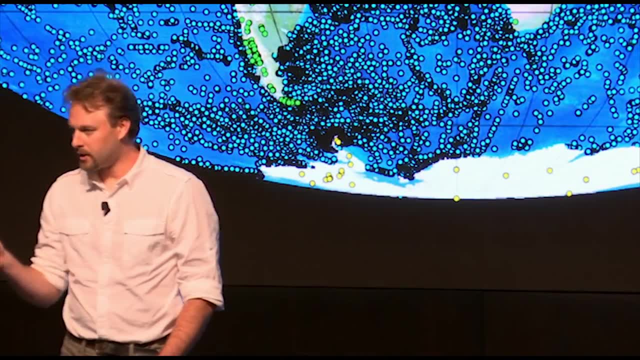 to do this And, for example, when we look at sediments, we might actually take out single organisms and look at the biology that exists, And sometimes we actually can take those organisms and run chemistry on them as well and understand the chemistry of them, And then you might need 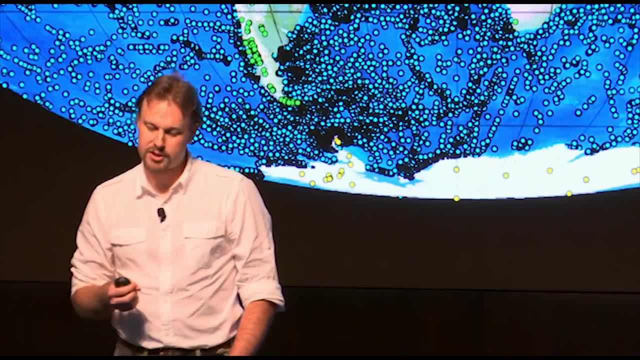 to know a little bit about how the ocean is mixing, and that's where the physics starts playing a role, And so all these different aspects are really important in trying to integrate this record, which becomes complicated, right? It's not an easy system, And you're. 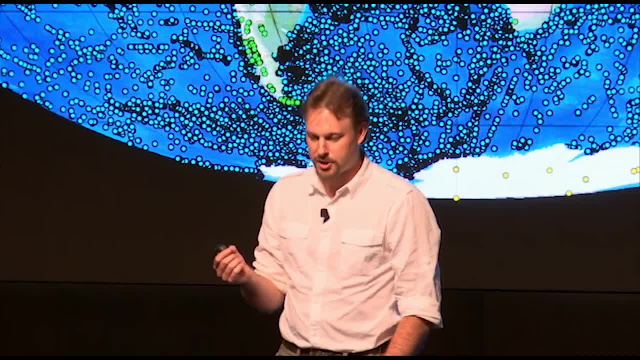 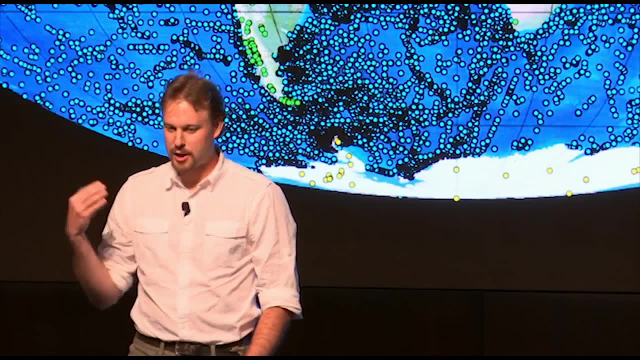 trying to put together how the Earth responds to different climate change. And so, over the time- we've been doing this for four years, we've been doing this for 40 or 50 years- we've gotten a much better idea right. That puzzle is becoming more. 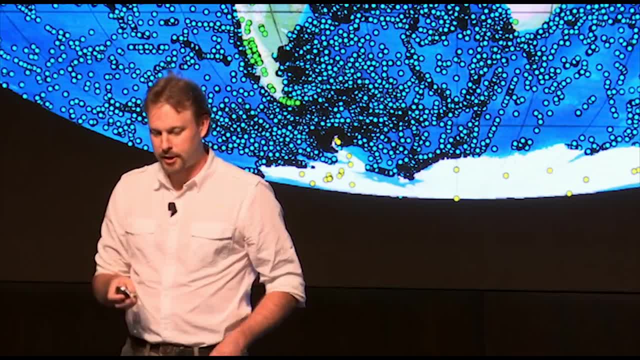 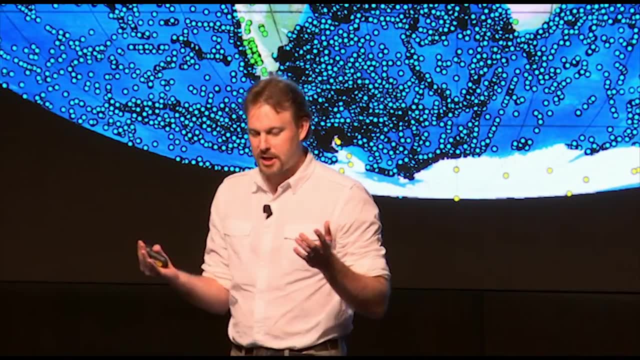 clear with the passing days, And so we're getting a better record, And so what we've really noticed is that you can take these different records and we can reconstruct CO2.. And so many of you guys might have seen glacial, interglacials, the last 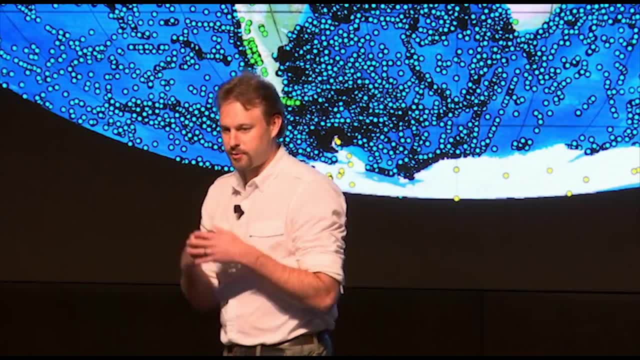 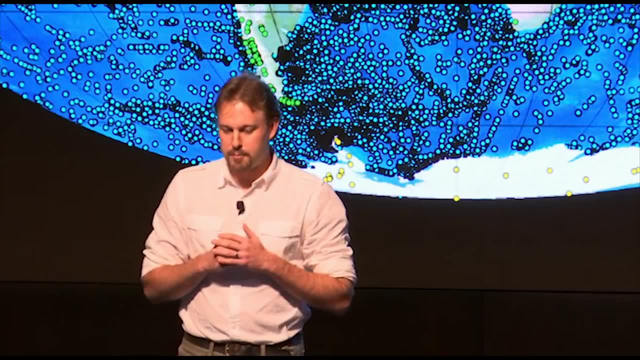 million-year record of temperature, where it's going up and down on a sort of 100,000-year record And with that we know temperature is also changing on about that time scale, And so these two things are different. They're definitely linked together. 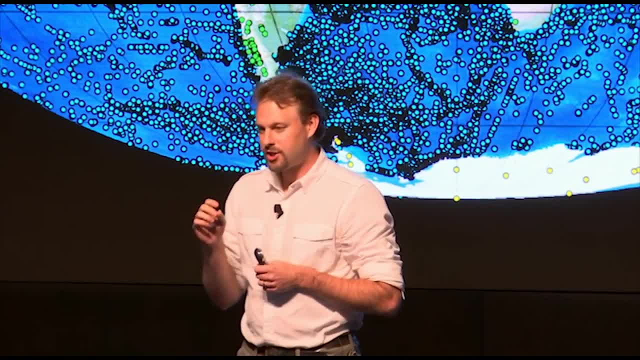 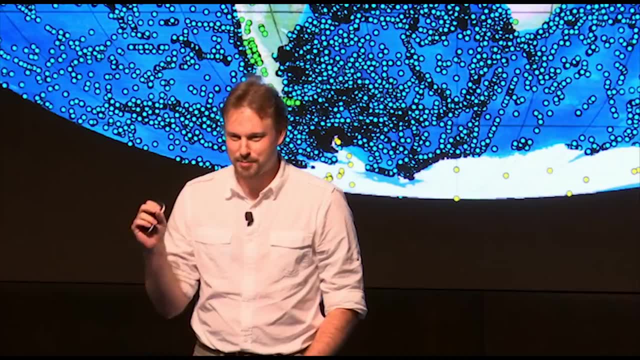 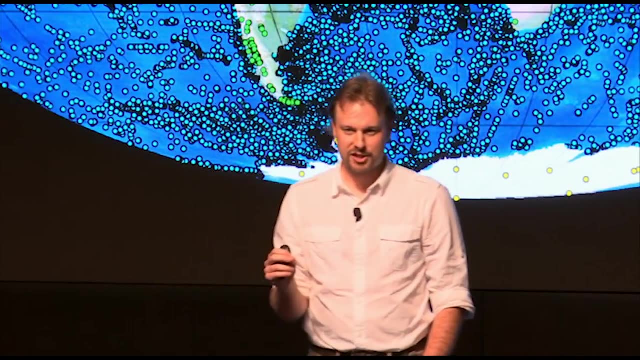 What we should really note is that the concentration change in CO2 over the glacial versus interglacial normal record is about 100 ppm. So I said that just previously, but we measured about 100 ppm change in about 60 years. What we're talking about when we talk about glacial, interglacial- 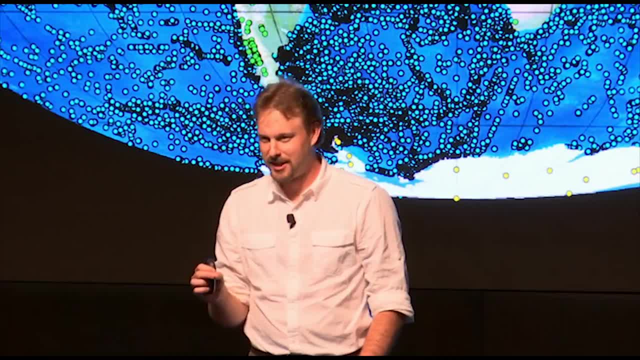 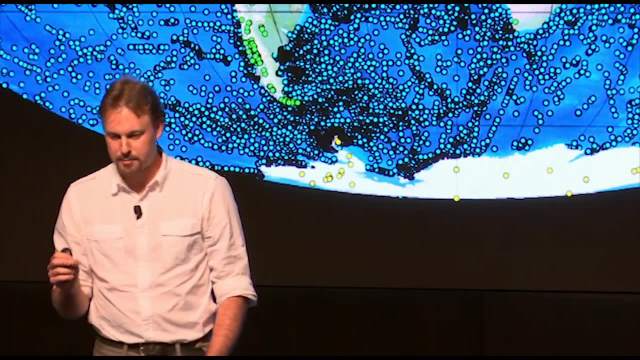 records is 100 ppm on hundreds of thousands of years right, And so there's a difference of about three and a half orders of magnitude difference on how fast this is changing, And that's a really important aspect. What I actually really am interested in is understanding how this might affect in the 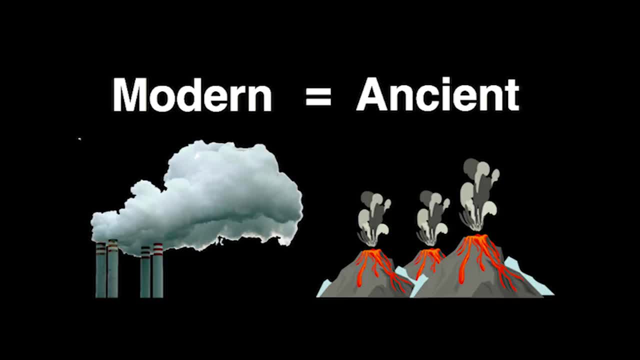 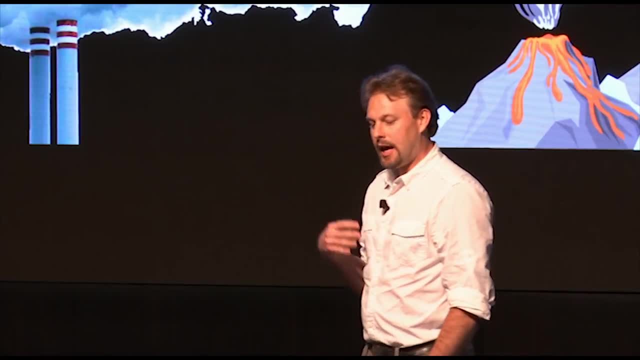 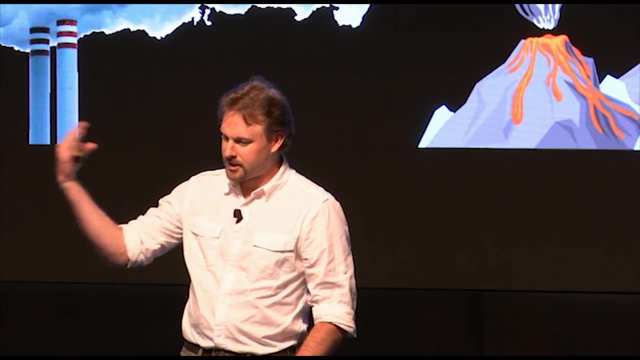 ancient record and what those changes might be. And so what is this telling us? is we study the ancient record to better understand what our future might look like and how the changes in CO2 might happen. And so you can think of the modern record as being sort of this anthropogenic release of CO2.. The ancient 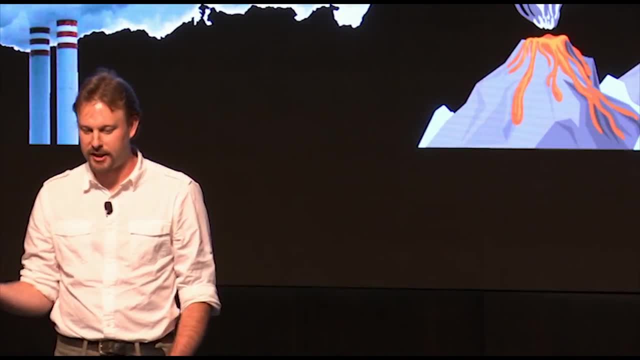 record. when we do this, we can only use basically volcanoes that release CO2.. We can only use them very rapidly. When I say very rapidly, I mean on geologic timescales. So it's very slow compared to the modern record. 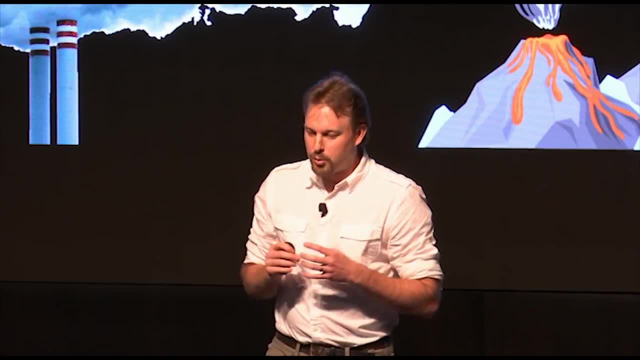 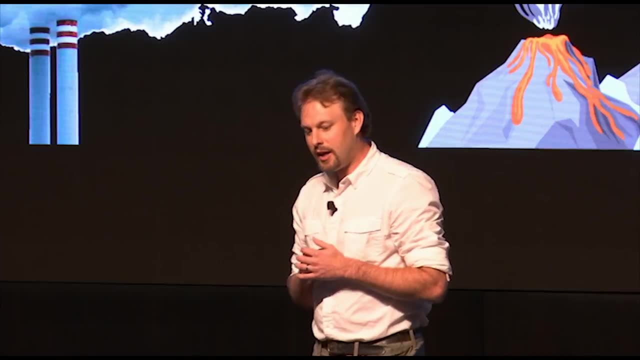 And so what we do is try to reconstruct this. Well, what we do have some ideas is we can have some predictable hypothesis, right? So with increased CO2, there's some predictions that you might make- You might have higher temperatures. Well, we see that today, right? 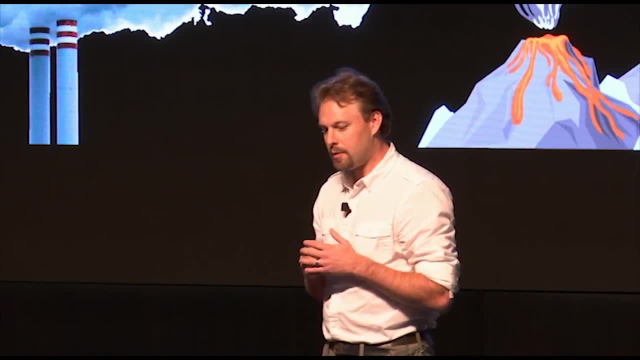 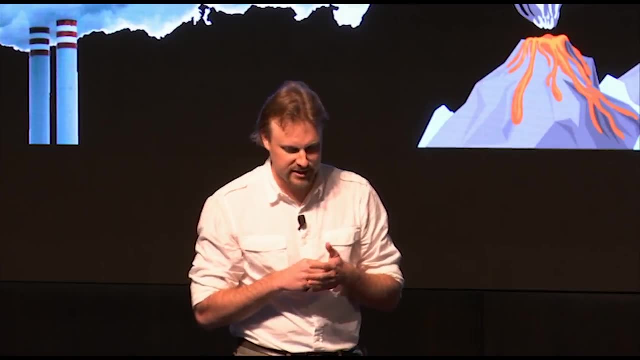 There also should be a sea level change. We're seeing sea level change- not nearly as fast, but it's certainly responding- and we're starting to see sea level rise, which is a big issue locally right in this state, And so those are two aspects that most people have heard. 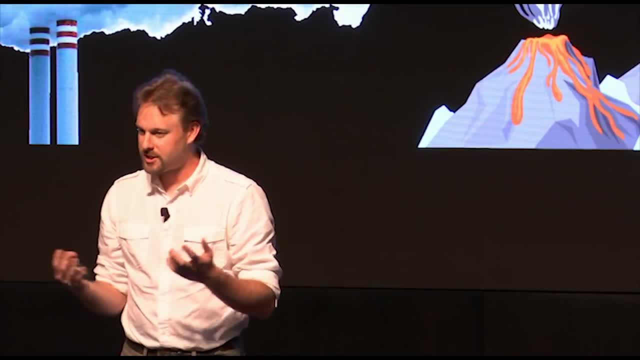 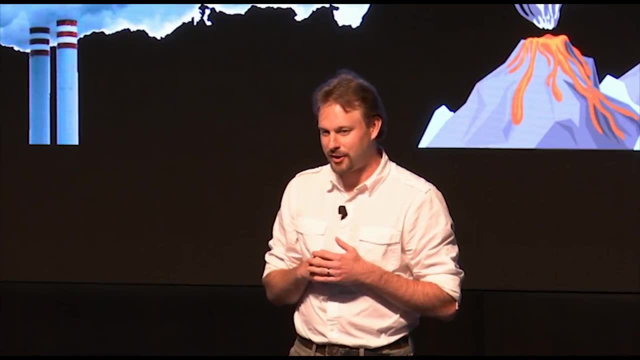 of Other things. we know that pH is changing, So pH we're getting more acidic. This is a really big effect on coral reefs, for instance, And so that's a major aspect. But one thing that you probably haven't heard of is oxygen, So we're actually seeing a decrease in oxygen. 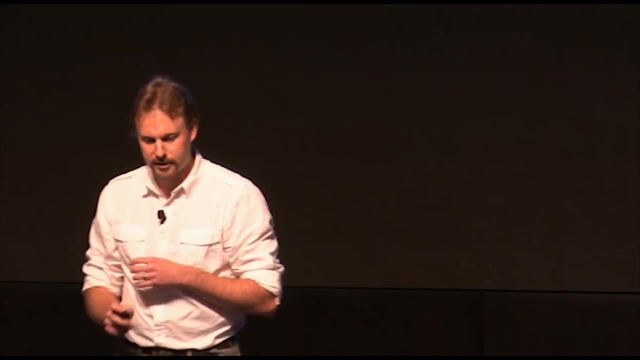 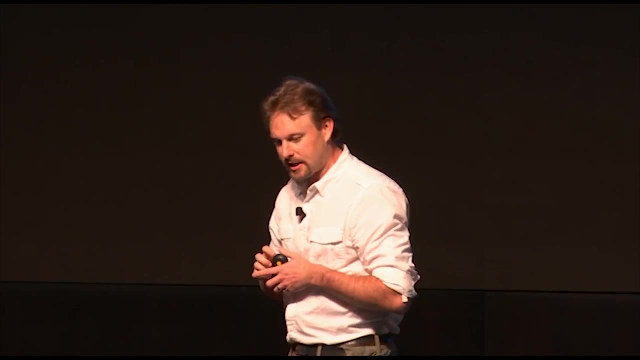 concentrations in our atmosphere and our oceans, which I'll talk about here in a second. So how does this sort of interrelated right? If you guys remember, sort of from a basic chemistry class, we probably have all seen this equation at one time or another, If we remember it, or 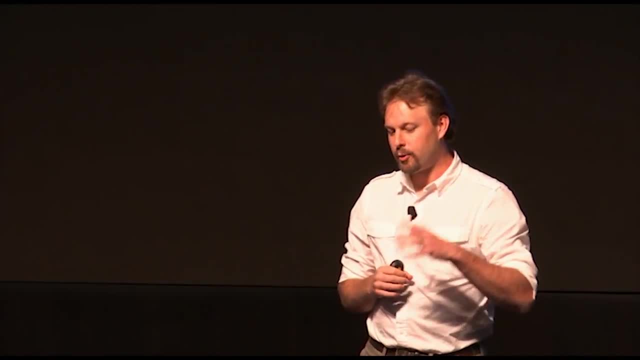 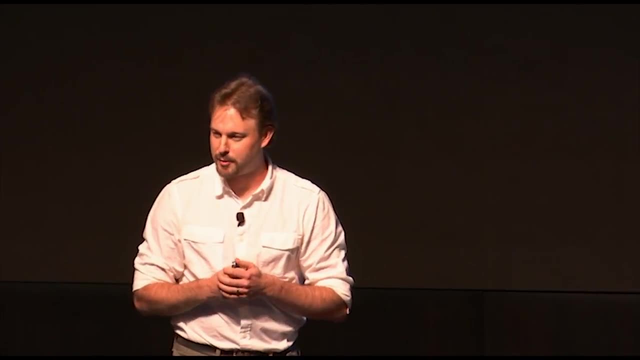 not, it might be different, But you can see going from left to right: organic matter and oxygen. This is what you and I do- Any other animals as well- right, We take up organic matter and oxygen and we get energy from this. So I can be up here speaking to you guys. 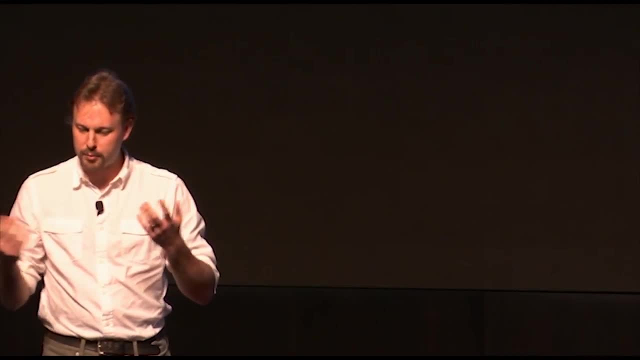 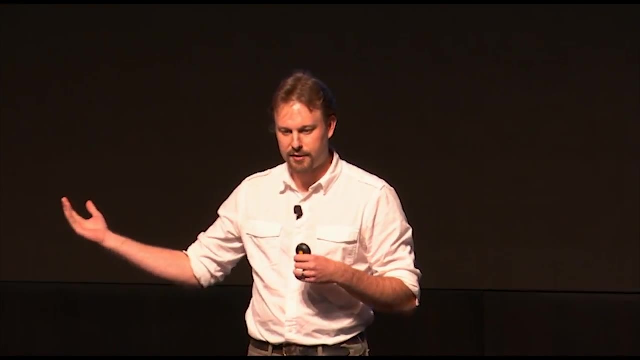 And we release CO2 and water vapor, And so that's what we are breathing out. And the last thing is: niedands are mutating Plants or primary producers. photosynthesizers are doing the exact opposite, So they are working from the equation from right to left. 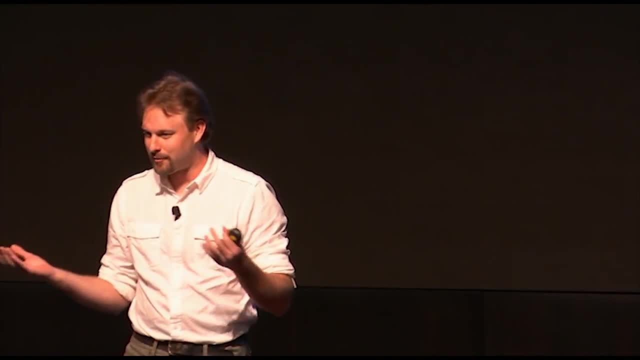 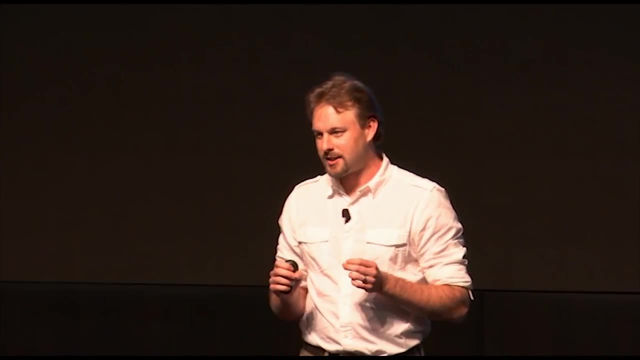 So they take water and CO2, make organic matter and oxygen, And so equilibrium. these things are not really changing right. They're balanced. But what we do when we burn fossil fuels is combustion, And you can think of combustion as being the exact same thing as respiration. 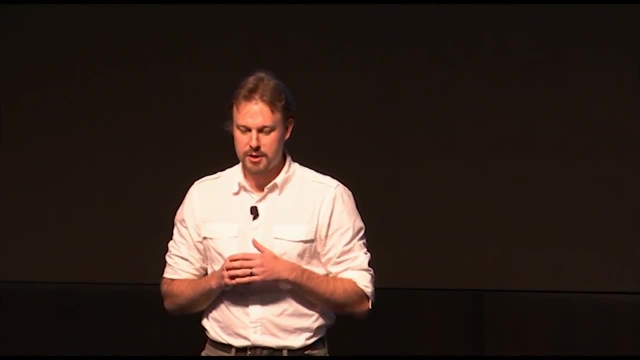 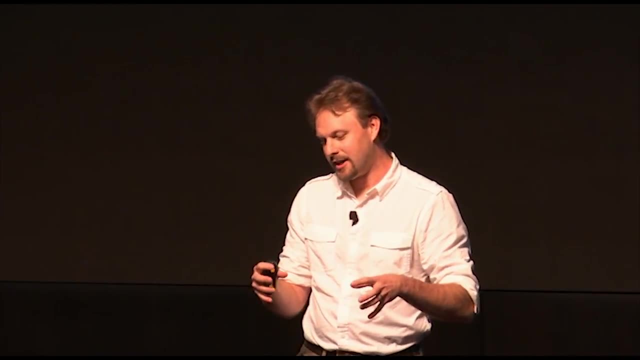 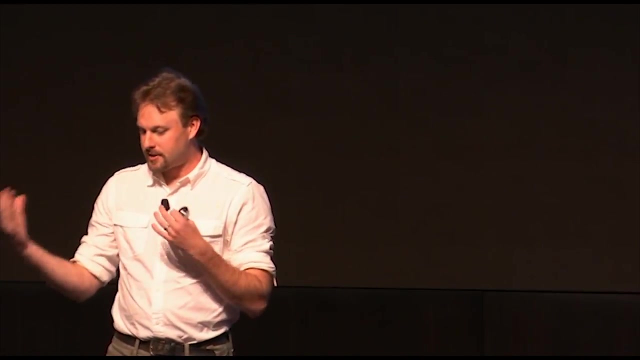 So chemically it's the same idea in the carbon emissions. And so the CO2 or organic matter that we take and put in our cars- fossil fuels, right. We combust that using oxygen in our motors and that then gets energy. we release CO2 and water. 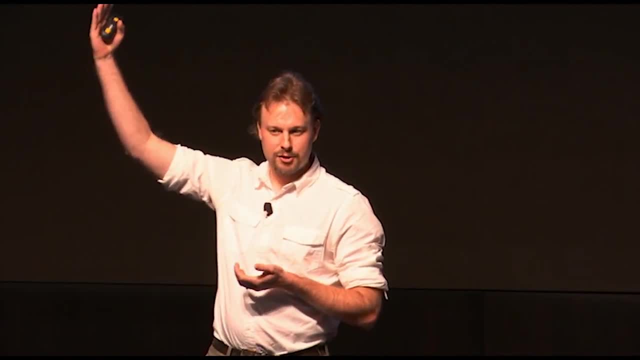 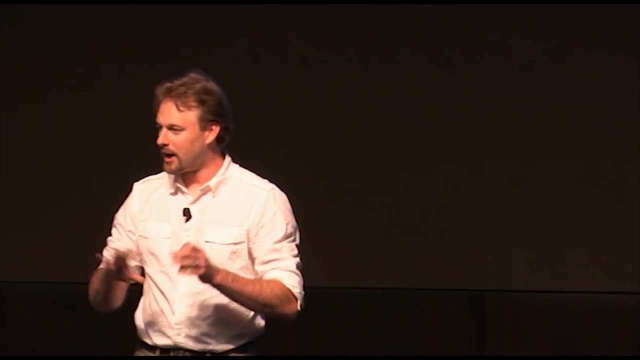 And so, if we're doing a lot of that, we would expect- and we see CO2 changing- we would expect oxygen decreases as well, And we actually see this, and this is one line of evidence that suggests that volcanoes are not really a big player in this. 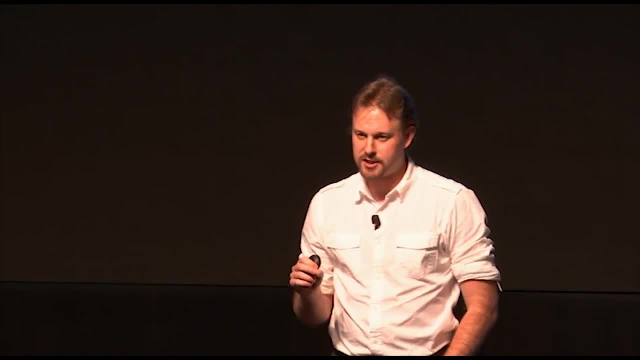 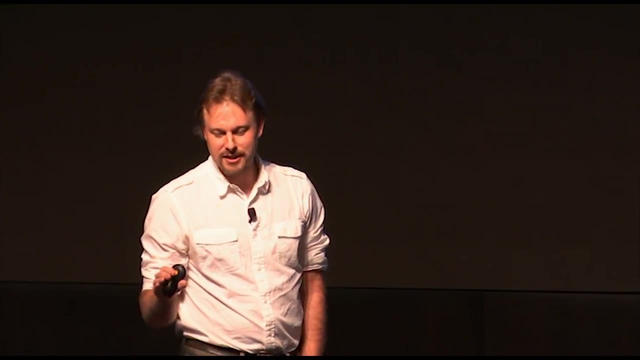 is that we actually can measure. in the last 15 years, oxygen decreases in our atmosphere. Now you might be going: oh my gosh, how is that going to affect us? We have a lot of oxygen relatively in our atmosphere. This is a really, really small difference. 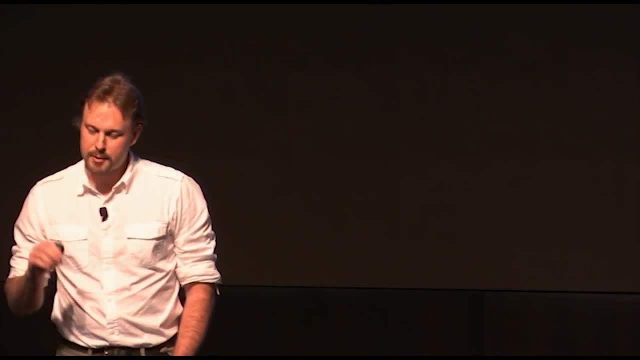 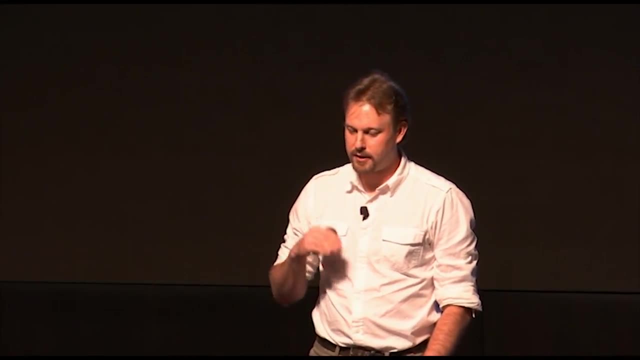 There's no harm to us at this point in our atmospheres, but we do measure a difference, and it's equal to the amount of CO2 that we're releasing, And so this is a really good line that this is really happening and it's anthropogenic or human induced. But what is probably a much bigger important player is that our oceans are becoming deoxygenated, And so over the last two decades, each decade we've lost about 1% of the oxygen out of our oceans, And that's not a huge amount. 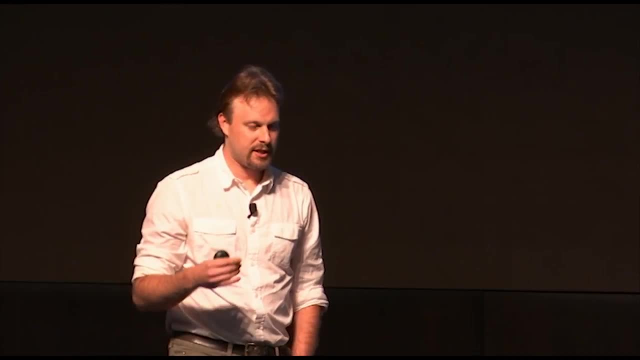 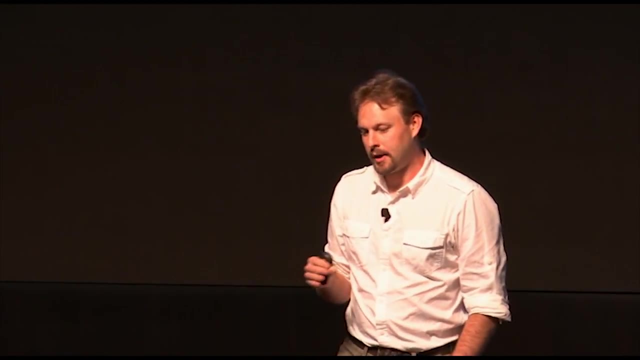 but it's enough to start really affecting things like fisheries and primary producers in our oceans and how that might respond, And so you can imagine, if you play this out for a while, what that might do to our ocean ecosystems, the chemistry and the biology. 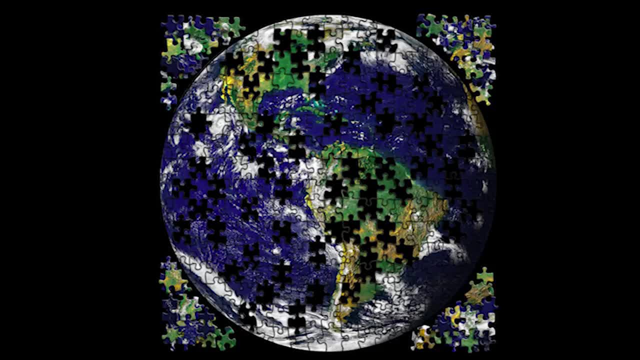 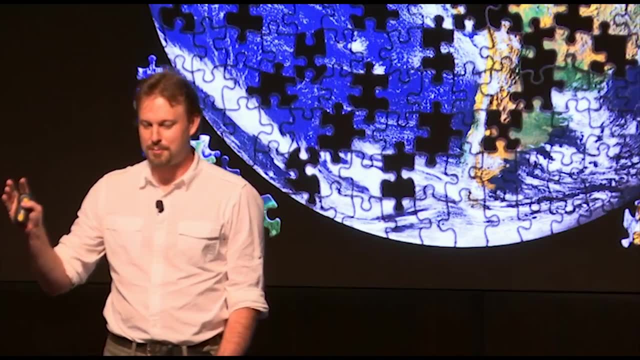 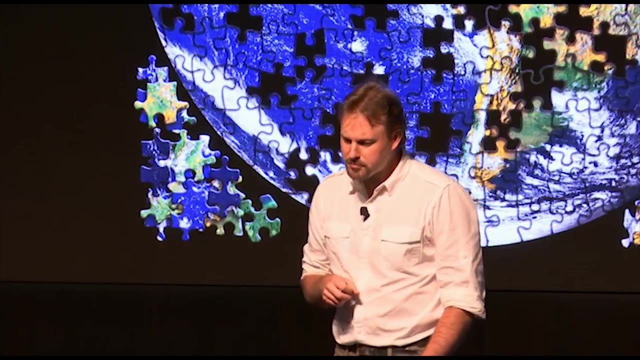 And so we are interested in my lab of understanding how oxygen has changed throughout Earth's history, And so you can imagine the puzzle of Earth. you get a lot less pieces the longer or farther back you work in geologic history, And so it does become difficult. 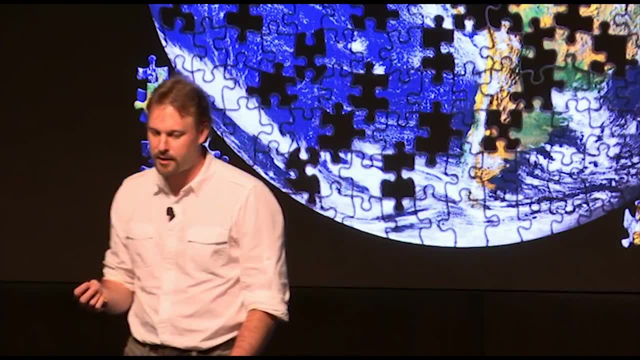 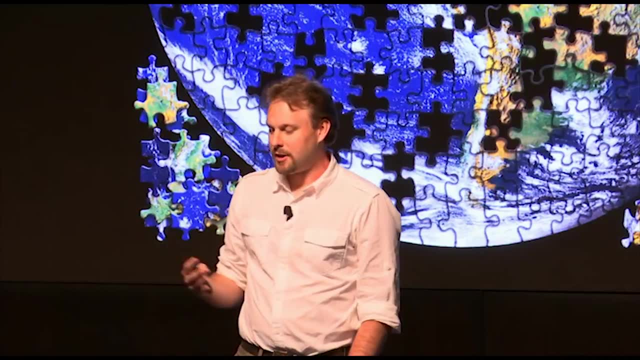 and there's certainly aspects that we can't explain or have a full understanding of, But you can see that we've removed about a quarter of the pieces out of this figure And you can still make out the large dominoes, And that's what we're trying to do. 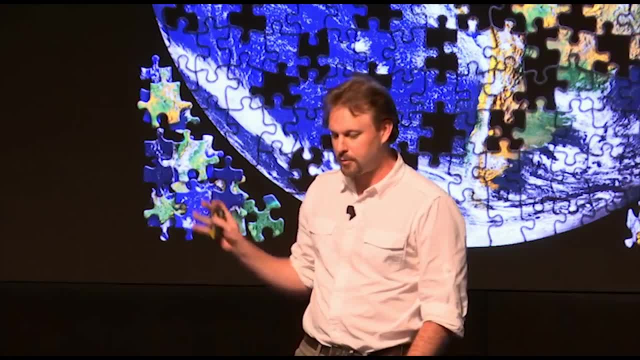 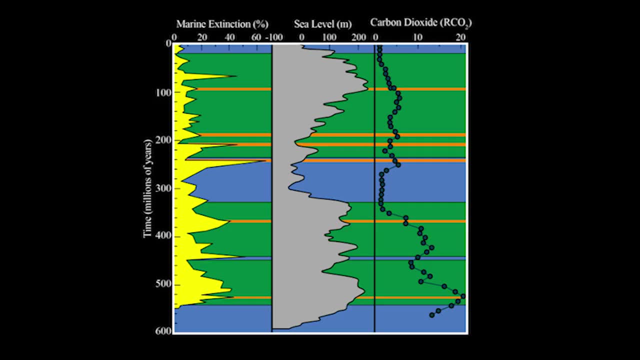 And we're trying to understand ancient climate change throughout geologic history And we are starting to get to paint a picture that we have a much better understanding of. And so with this, this is a relatively complicated figure, but this is the last 600 million years. 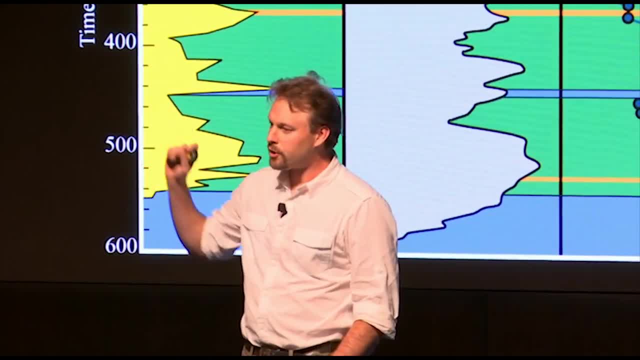 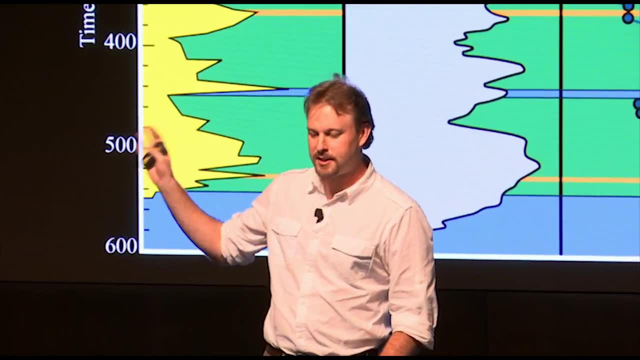 which has went since we've had animals on this planet, And the blue bars represent time periods of glaciations. So these are major glaciations, similar today. It means you have ice at your polar regions And you can see that doesn't make up a large amount. 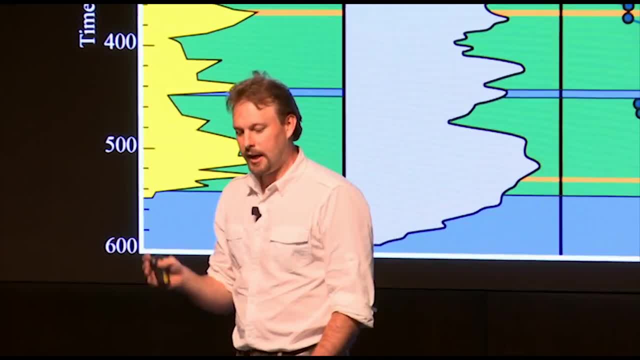 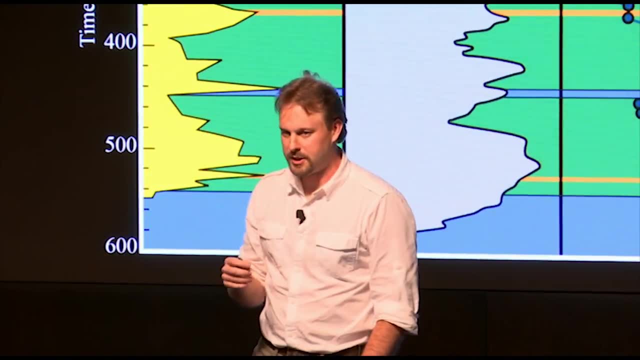 of Earth's history. they are time periods when both sea level and carbon dioxide are a little bit lower, And then the time periods in green are greenhouse events. So this would be similar to when the dinosaurs were around. You have no glaciations. 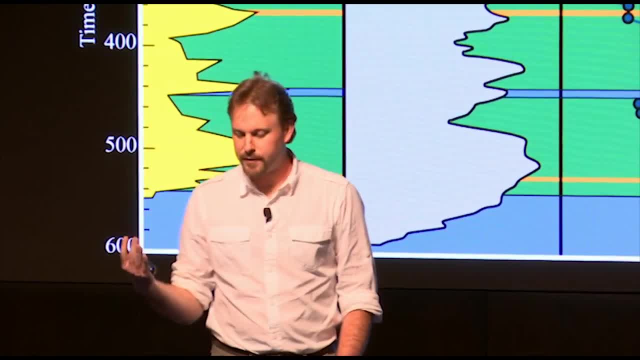 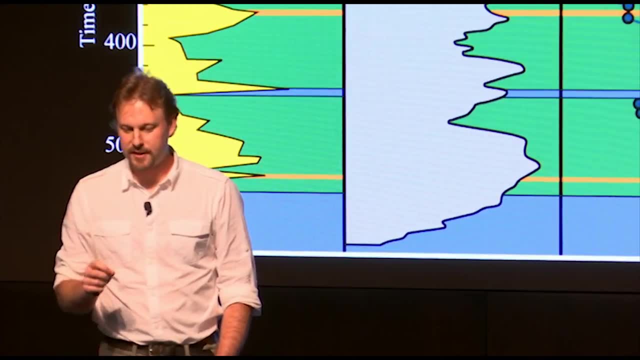 even sometimes palm fronds in the polar regions, And so very warm, high sea levels, higher CO2.. And what I want to point out here is that the orange bars are places that we can definitively say that there's a reduced amount of oxygen in the oceans. 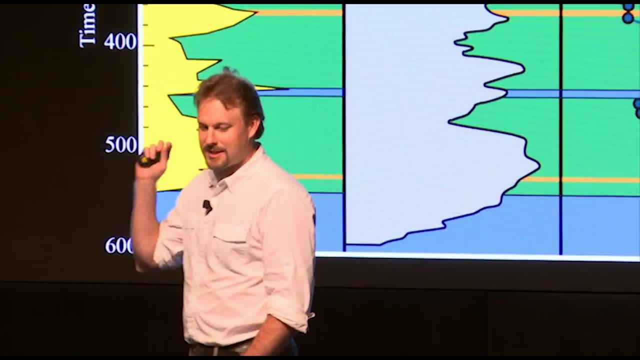 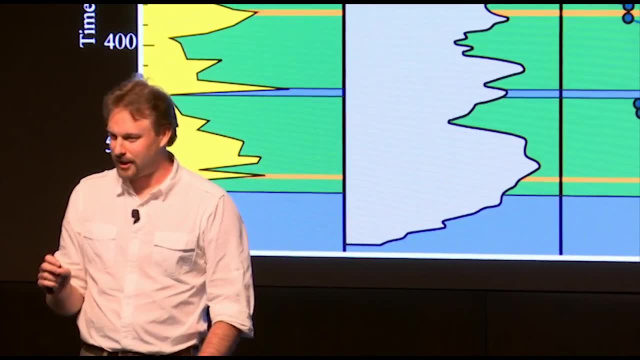 Very, very small amounts of oxygen And they relate almost entirely to every extinction event that we have so far looked at right, And so the extinction events that we see all are related to some sort of deoxygenation or climate change in general. 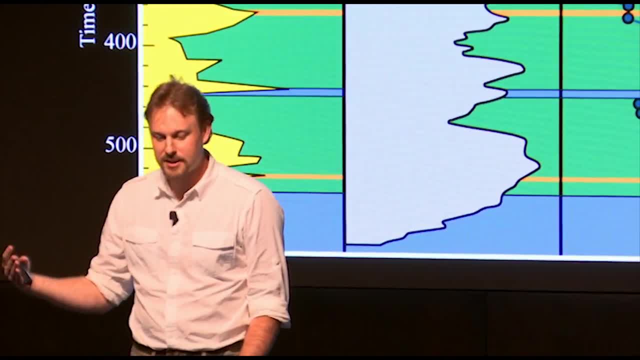 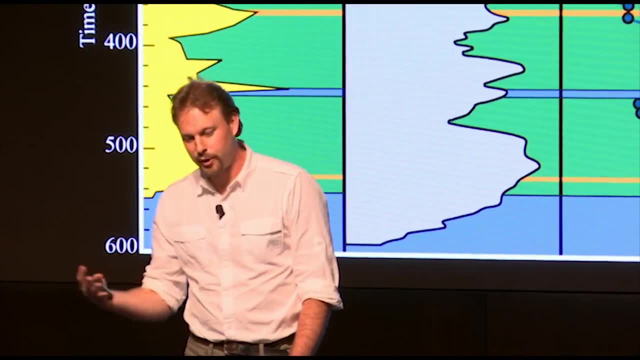 And so this becomes really important of how quickly is this happening And can this be a major important effect that might happen in our future if we don't sort of slow down climate change and make some changes? And so this is a really important fact. 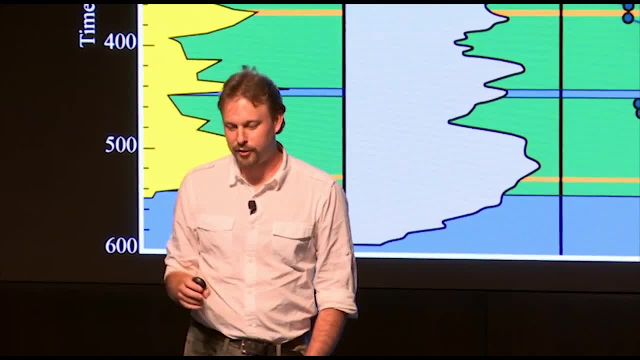 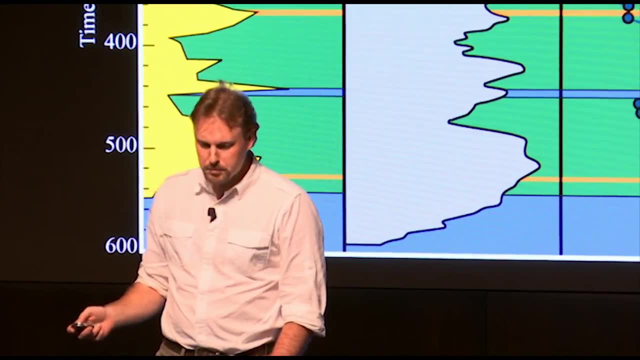 We're probably not headed there Like tomorrow or any time in maybe even our lifetimes, But certainly in terms of thinking of the earth and how it responds, this becomes really important, And so there are some solutions. right? This sounds kind of doom and gloom. 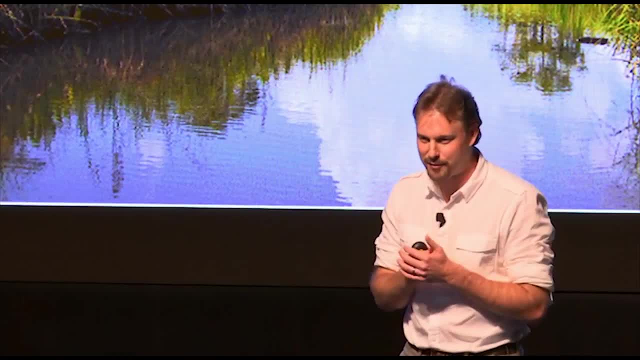 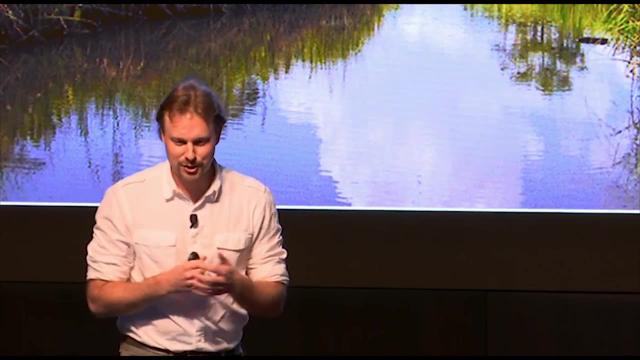 and everybody always sort of ices over when we talk about climate change, just because it does sound really scary. These are usually long-term changes, but what we do have is some solutions. The obvious solution is reduce our CO2 emissions or our carbon dioxide. 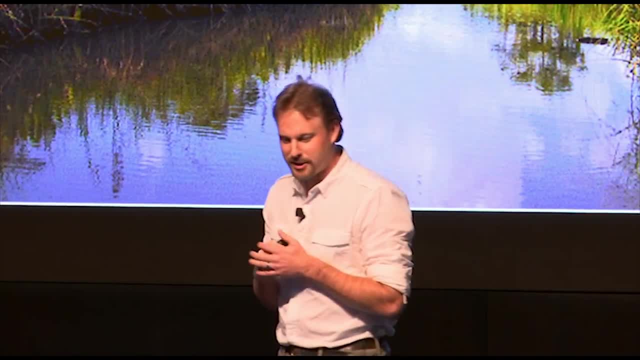 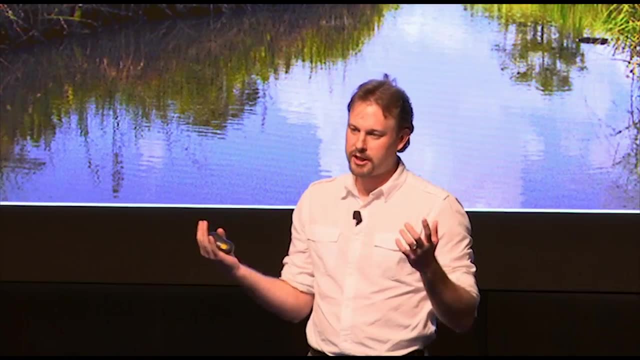 And that's easier said than done. right, Probably all of us are still going to use electricity. I'm going to drive my vehicle when I go home as well, But there are other types of solutions and certainly community solutions, And here in Florida what I would like to really drive home. 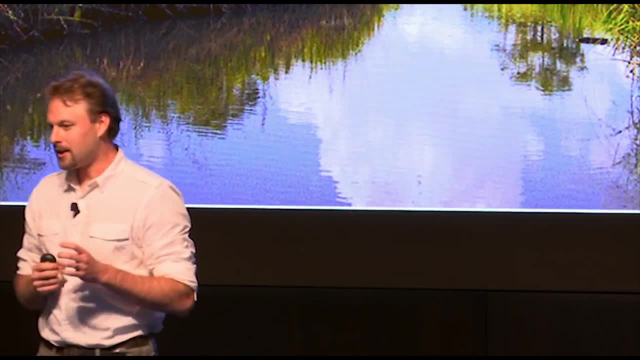 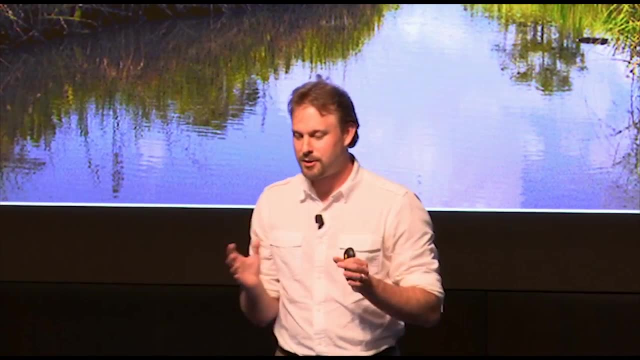 is that one of our major solutions is protecting certain types of lands, And those are estuaries and marshlands, so sort of coastal regions, And so if we can reduce the amount of, let's say, building on these environments or getting rid of them entirely, we will actually